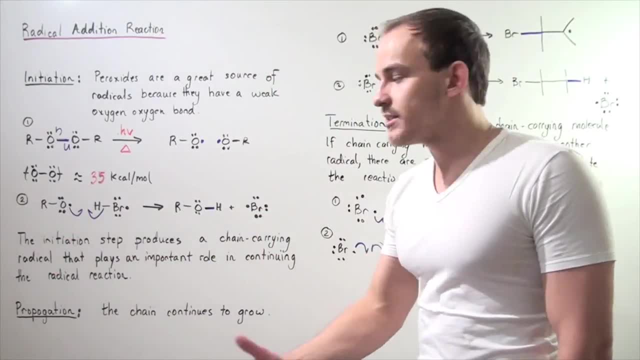 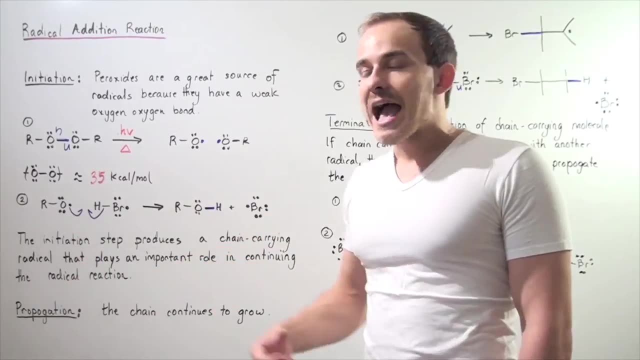 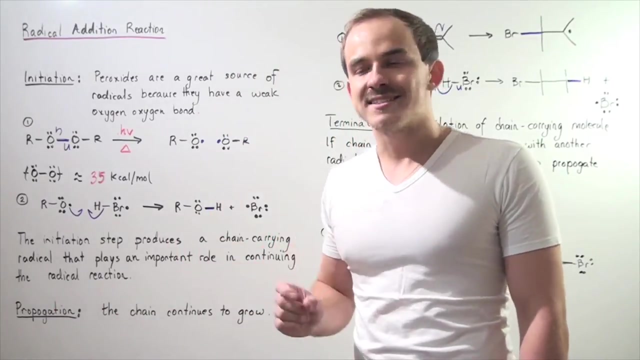 So, once again, the initiation step produces a chain-carrying radical and this radical plays a role in propagating our radical reaction. And now we jump directly to the propagation step. This is our second step in which this chain-carrying radical is going to be propagating. 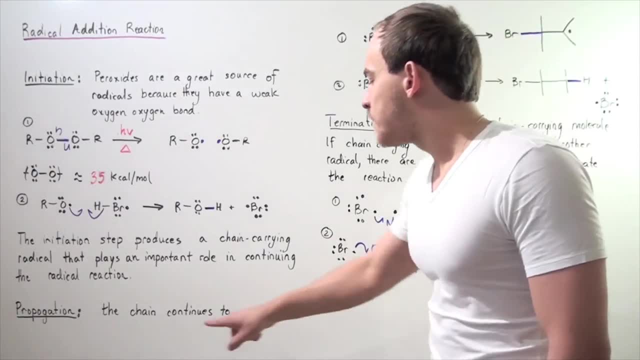 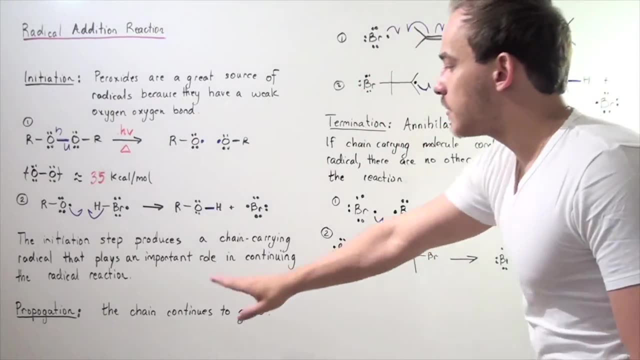 This is our second step in which this chain-carrying radical is going to be propagating. radical plays a role in continuing or allowing our chain to grow. So let's look at the two steps of the propagation step. What we have is an alkene reacts with a bromine, the chain carrying. 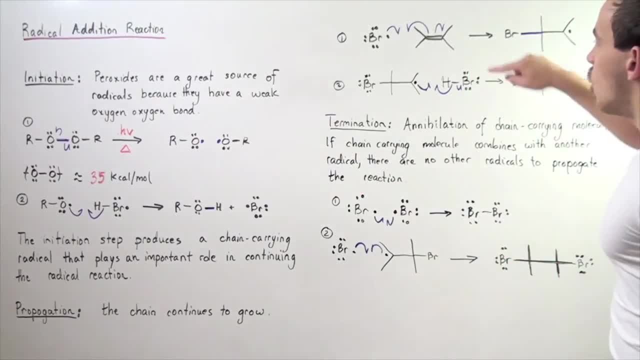 molecule formed in an initiation step. One of the electrons in the pi bond breaks off and reacts with this electron, forming the following sigma bond: And the second electron stays on this sp2 hybridized carbon, So that electron is found in a 2p orbital In the second step of the propagation. 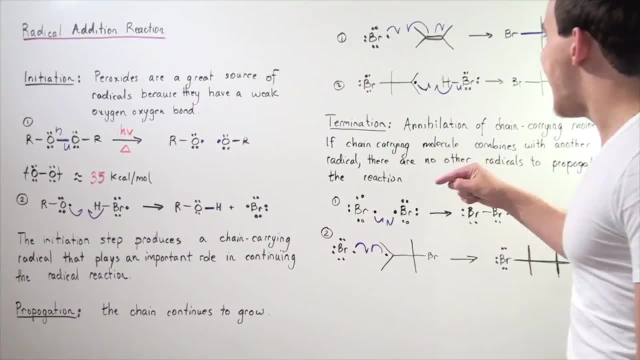 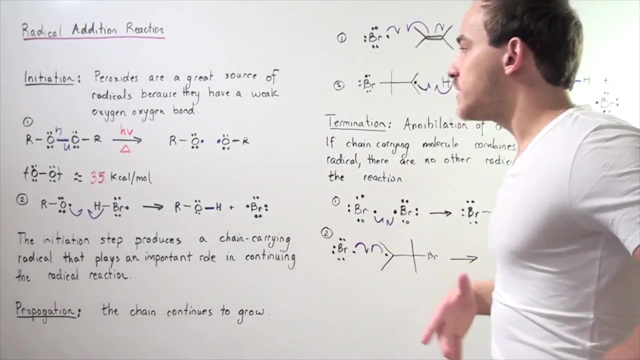 step, we have a second HBr molecule that adds to the product of this first step in the following manner: And we form the following: halogen-containing hydrocarbon and another chain-carrying radical. So we're essentially forming a chain-carrying radical. 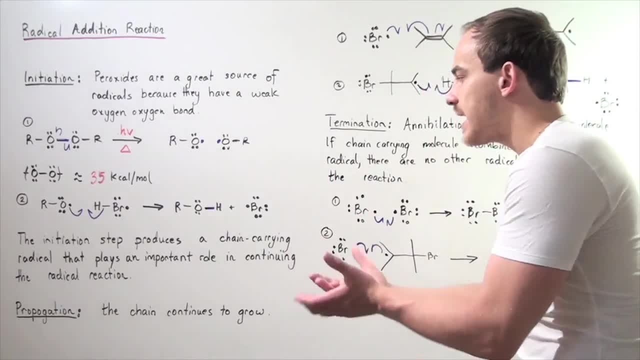 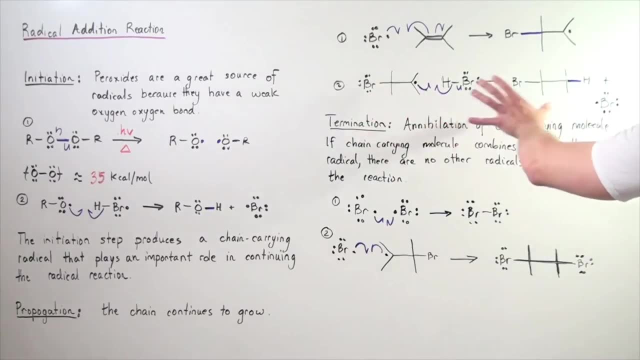 in the initiation step and we're reforming that same chain-carrying radical in our second step of the propagation step. Now, this reaction can continue until termination takes place. Termination is the final step. It's the annihilation of a chain-carrying radical. In other words, 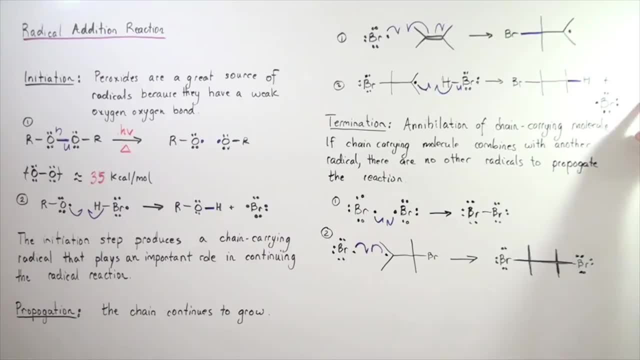 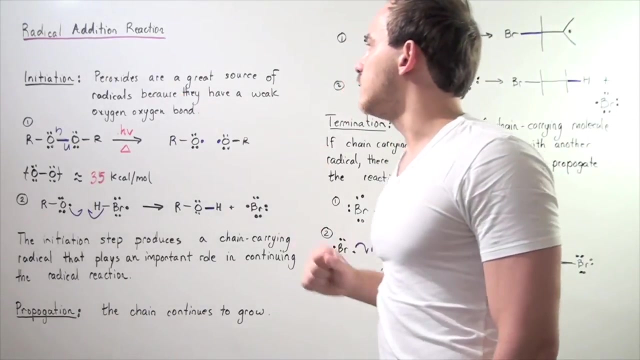 what happens is that this molecule, this radical, reacts with a second radical in an exothermic fashion to produce some molecule that's no longer a radical, And since we have no more radicals, we terminate our radical addition reaction. So let's look at the following examples Now. if this bromine radical, 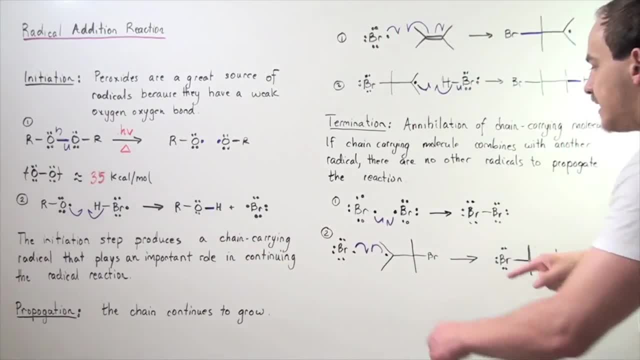 reacts with a second bromine radical. in the following exothermic reaction we get the following bromide or diatomic bromine, And now we no longer have any radicals. so our radical reaction is complete In a second type of termination step, this same chain-carrying radical.